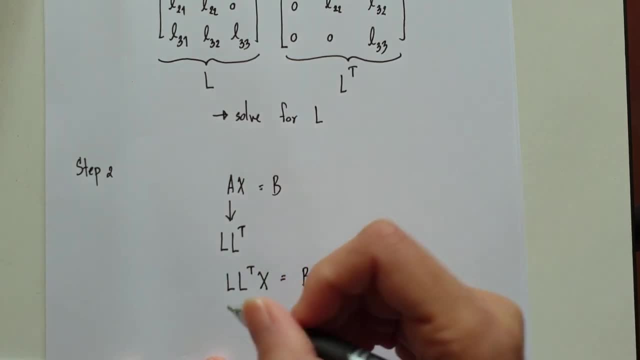 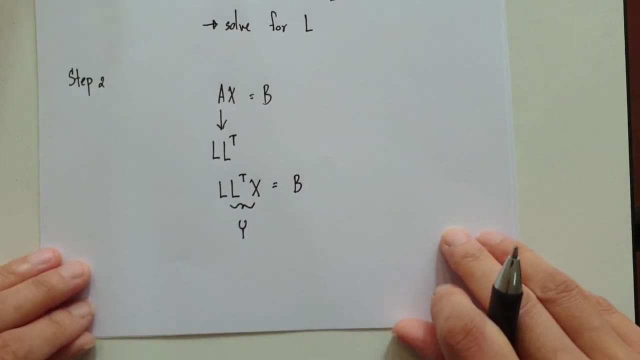 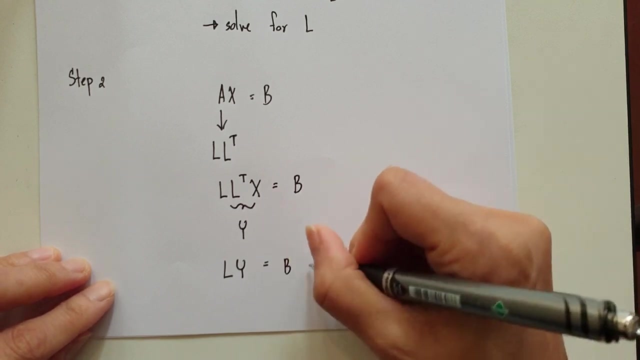 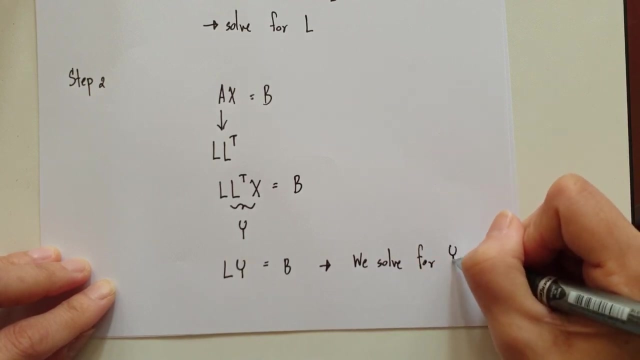 X would equal to B, And here we can set L, time, L, transport X as Y. So in the step 2, what do we solve? is L Y equal to B? Here we solve for Y. Okay, In the last step. This is step 2.. 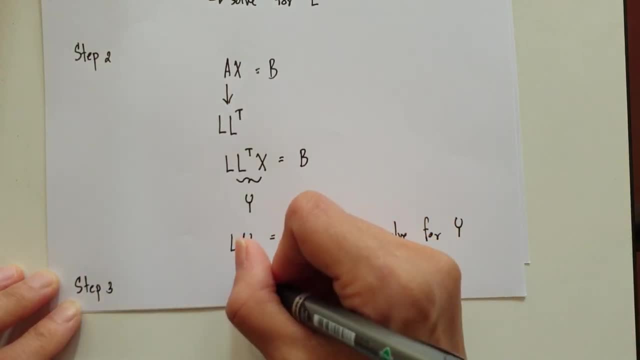 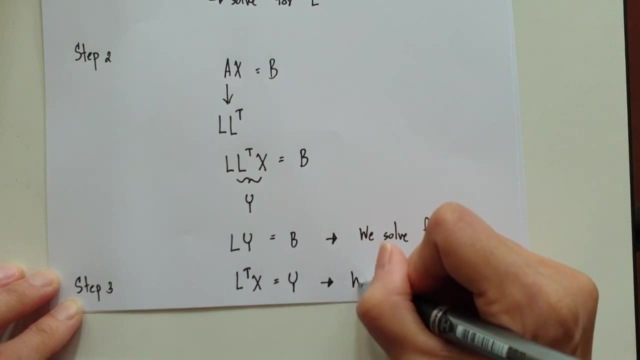 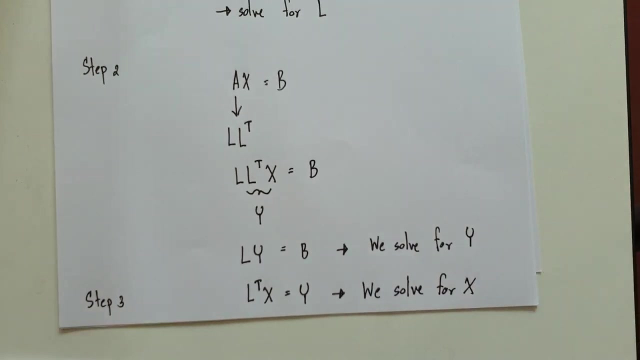 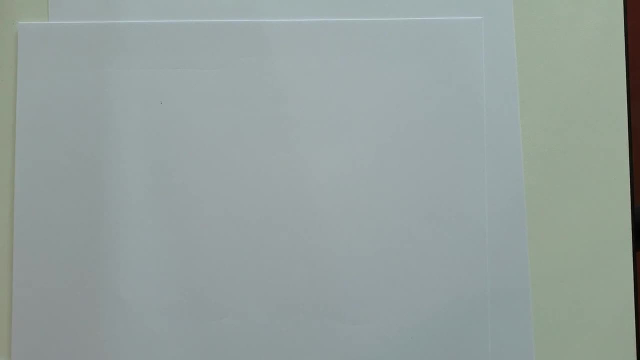 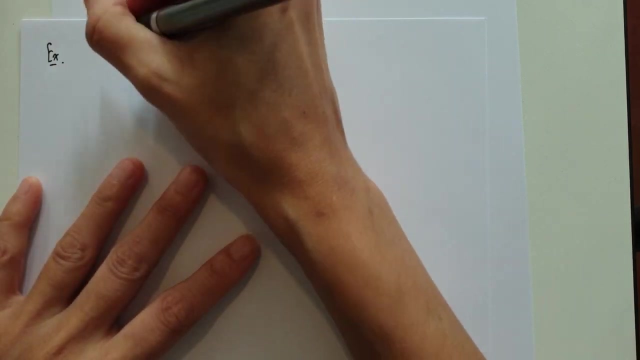 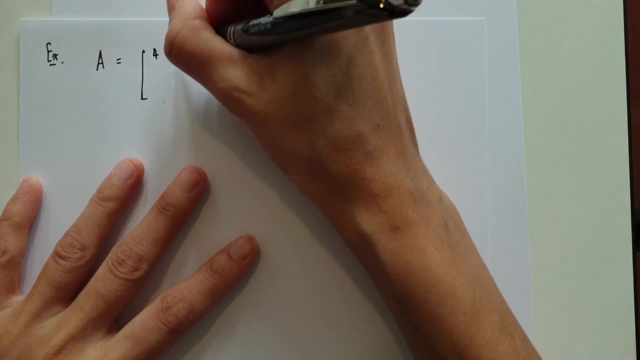 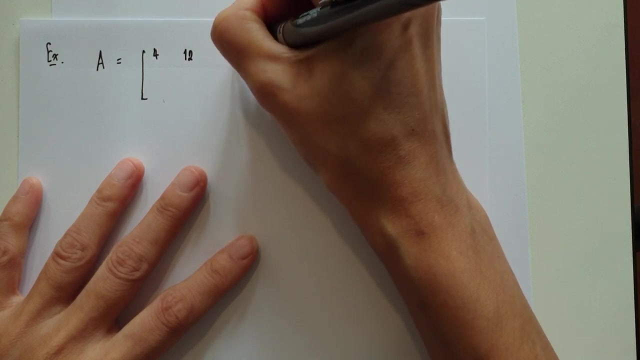 is the is the way. how do we find the matrix L? So I search in the internet and there is an example that they gave A as metric like 412 minus 16.. 12, 27 minus 43.. minus 43.. 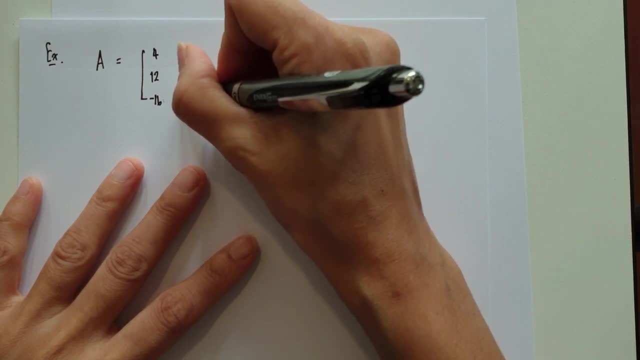 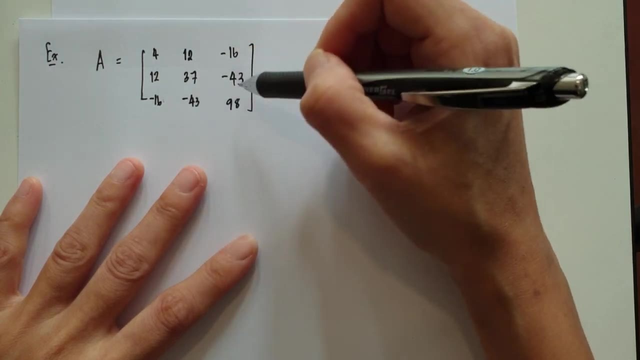 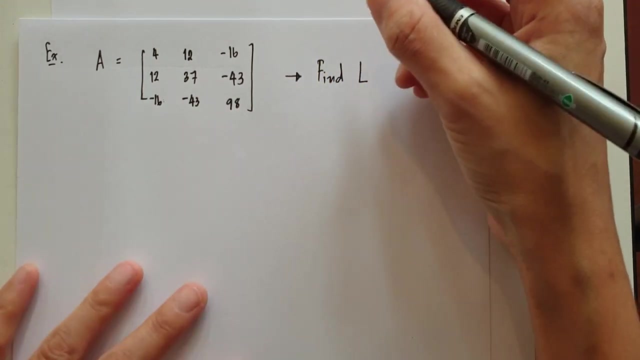 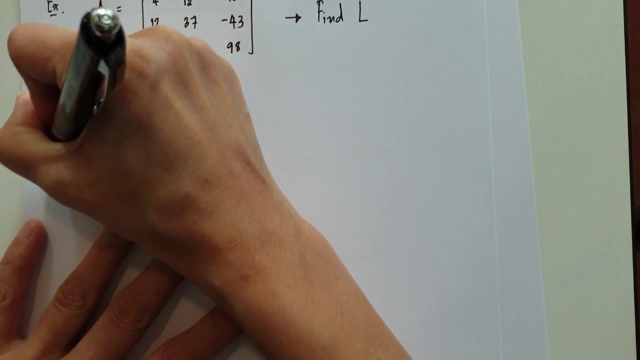 43, minus 16, minus 43,, 98,. okay, this is the symmetric matrix, right? so we will try to find L, okay, in this example first step. right? so what we will do is L11, 0, 0,. 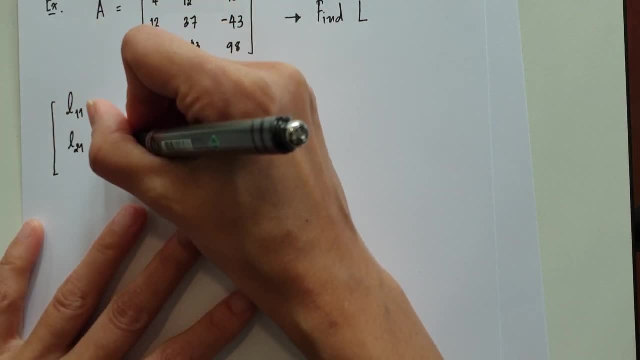 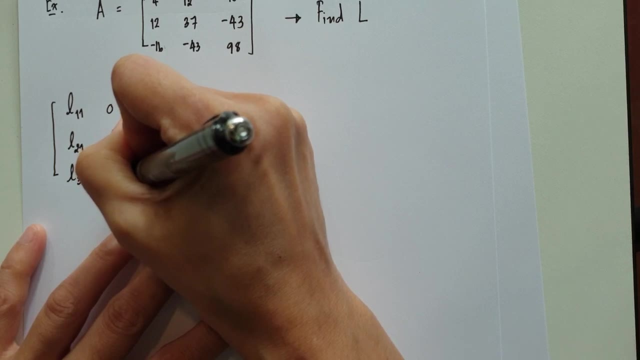 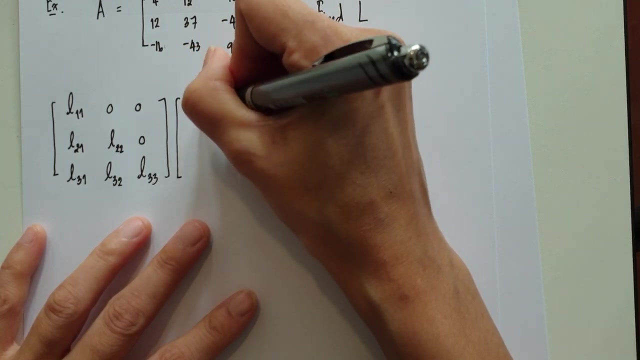 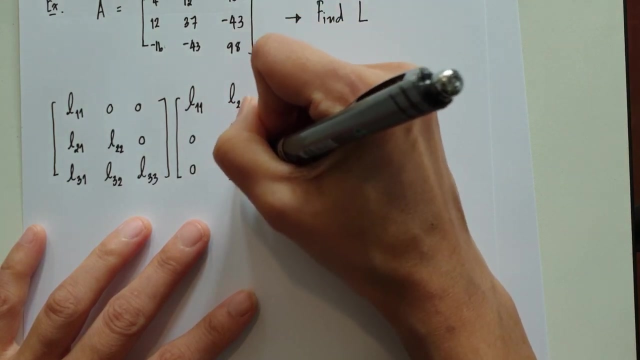 L21, L22, 0, L31,, L32, L33 times with L transport, which is L11, 0, 0, L21,, L22, L. oh sorry, this is 0, and here is L21. 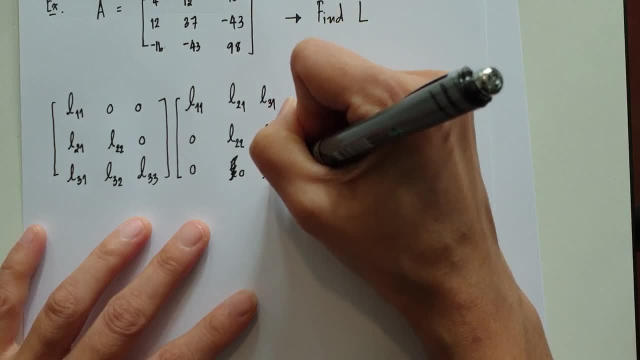 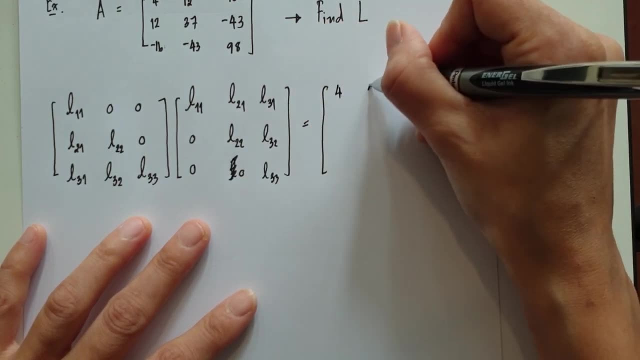 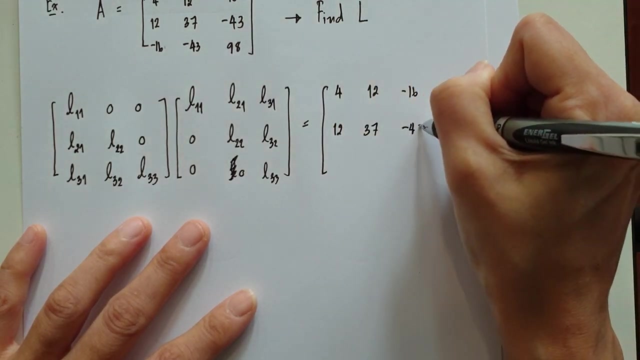 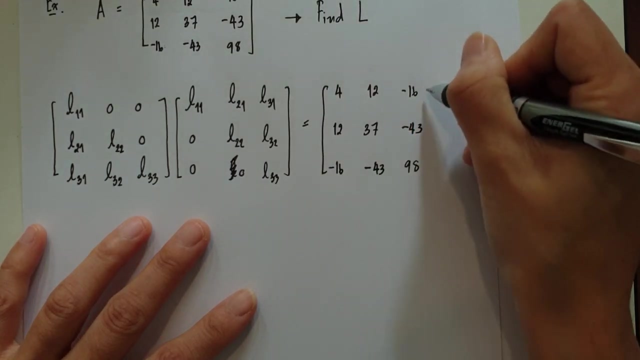 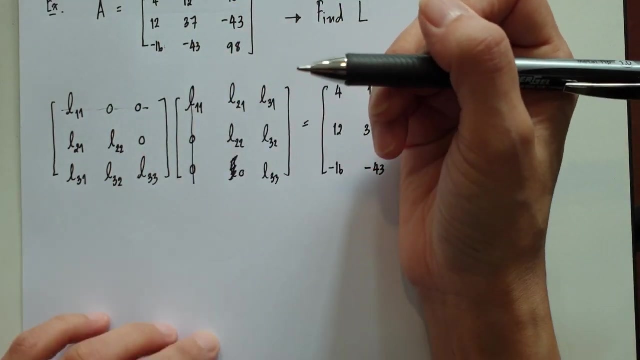 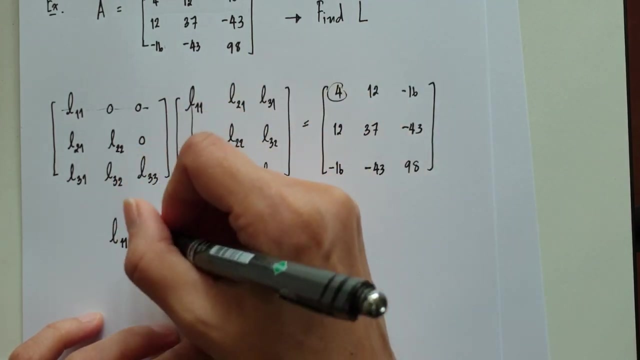 L31,, L32,, L33, right, and it would equal to A, okay, okay. so if we try to multiply the first row With the first column, we got 4, right. so from here, L11 squared would equal to 4, so. 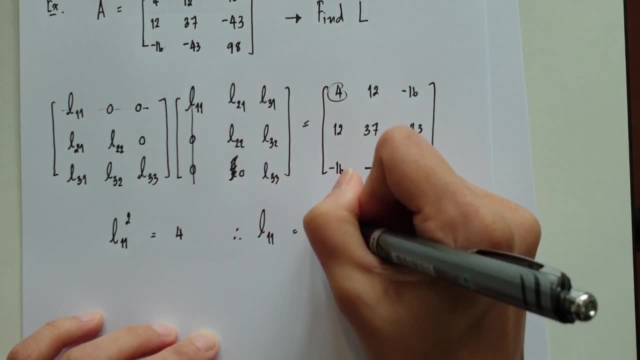 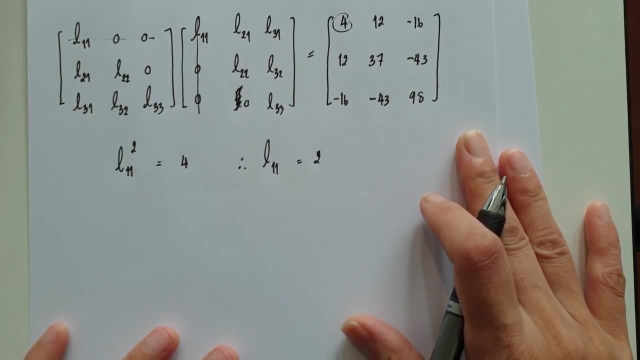 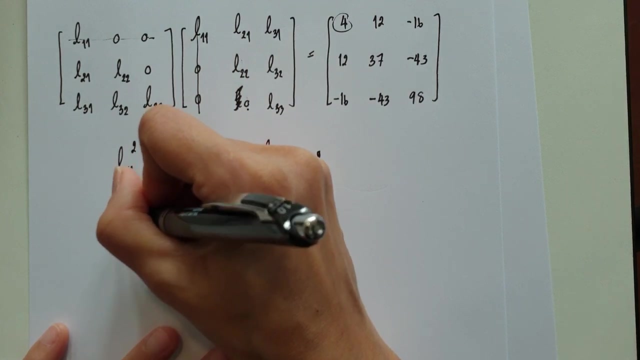 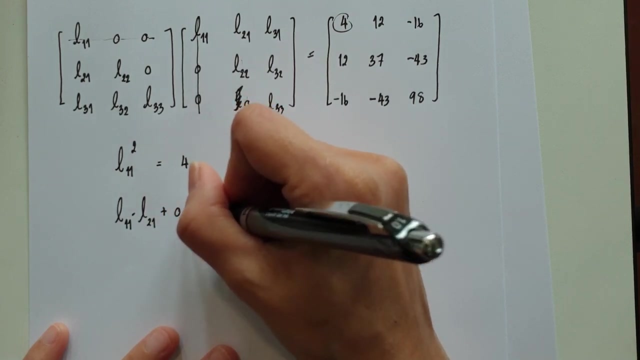 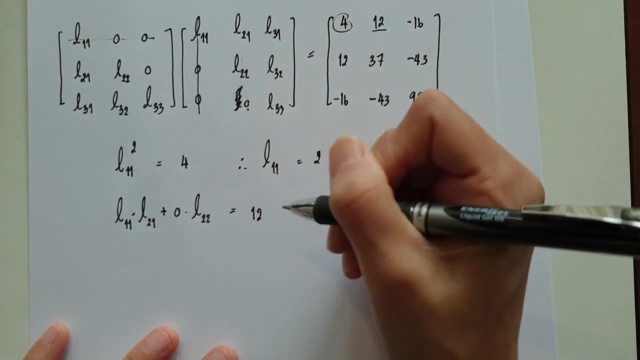 L11 would equal to 2,. okay. the next, we can multiply the first row with the second column, okay, Okay. so this is L11, L21 plus 0 times L22 plus 0, equal to 12, okay, so from here, L11. 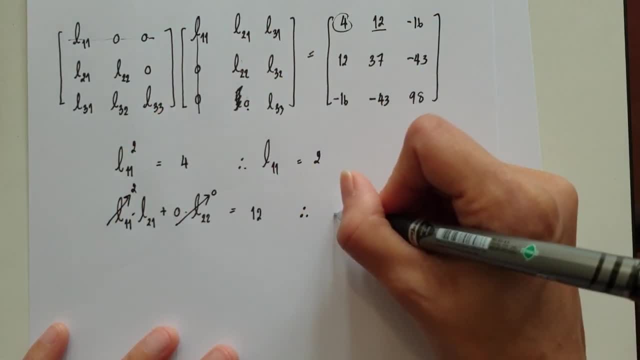 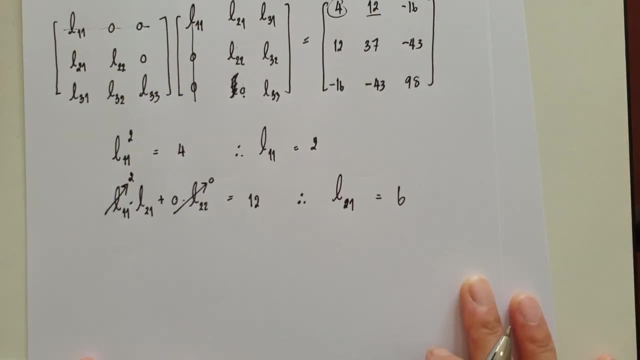 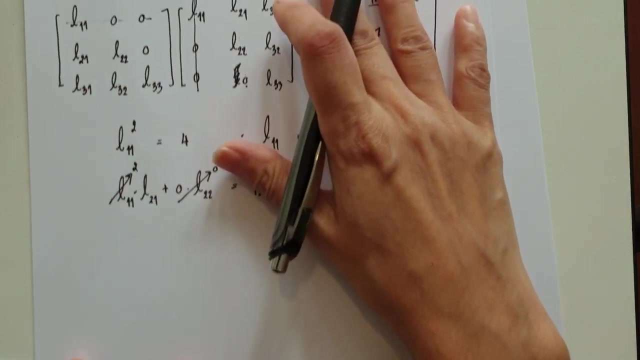 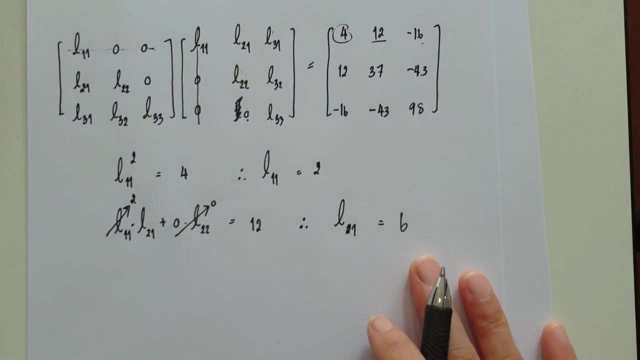 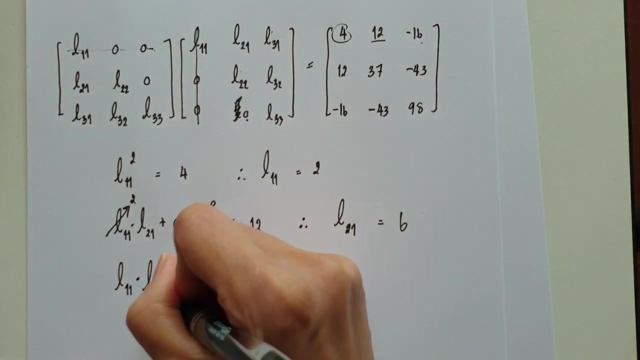 is 2,. okay, so from here, L21 would equal to 6.. L21 would equal to 6.. L21 would equal to 7.. Okay, All right. And the next is: if we multiply first row here with the third column, we got minus 16.. So this is: L11 times L31 would equal to minus 16.. 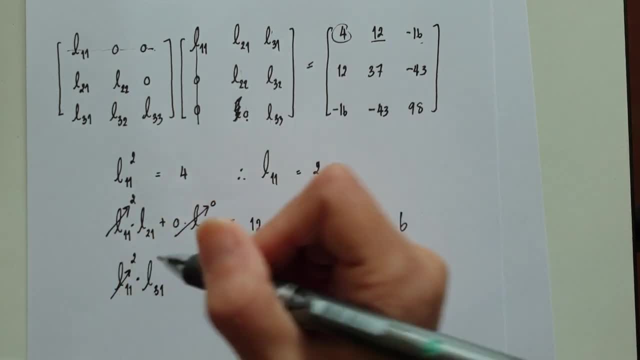 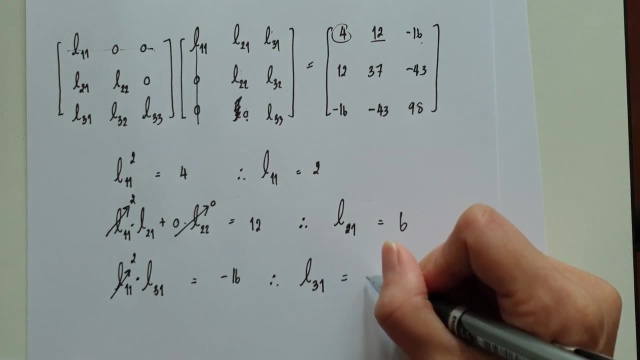 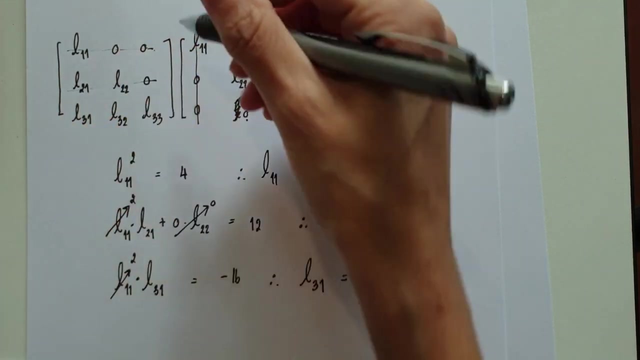 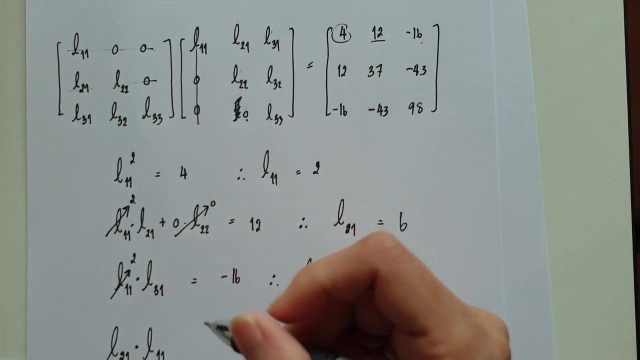 All right, And L11 is equal to 2.. So from here, L31 is equal to minus 8.. All right, And the next we move to the second row, start with the first row. So here is L21 times L11 would equal to 12.. 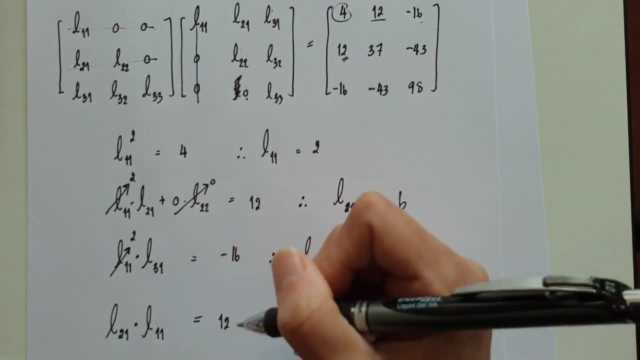 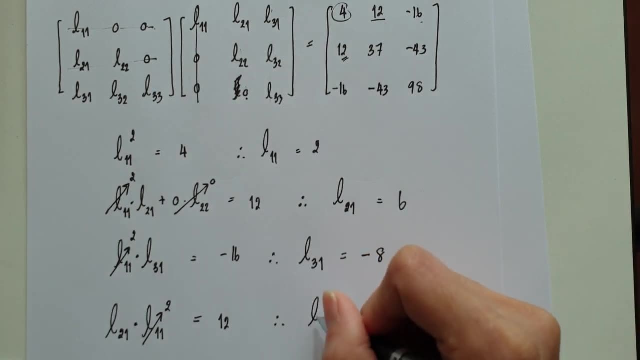 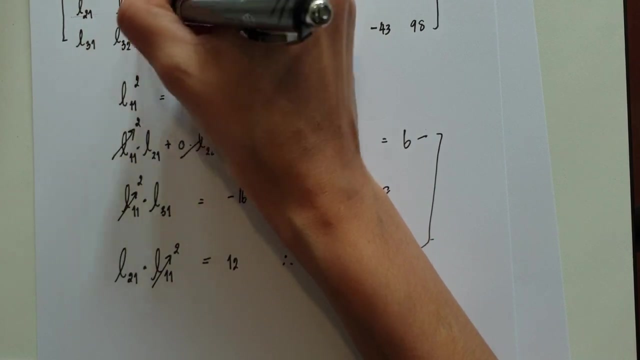 Okay, And L11 is basically 2.. So L21 is 6.. Oh sorry, This is a symmetrical matrix. I forgot. So almost the same, right. So what we can do is we can move to the next column. 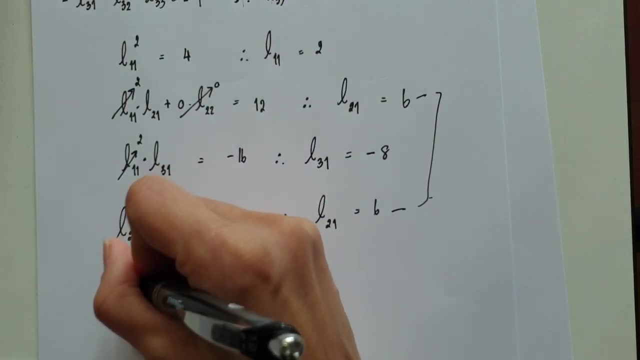 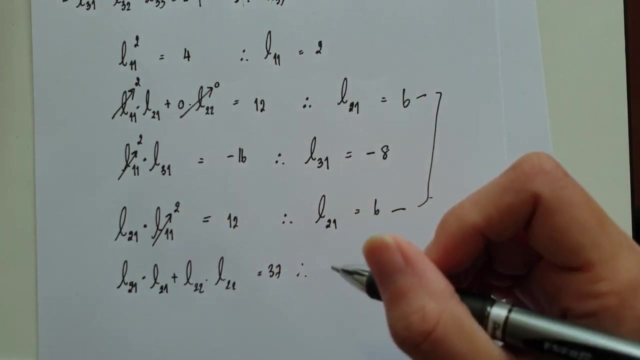 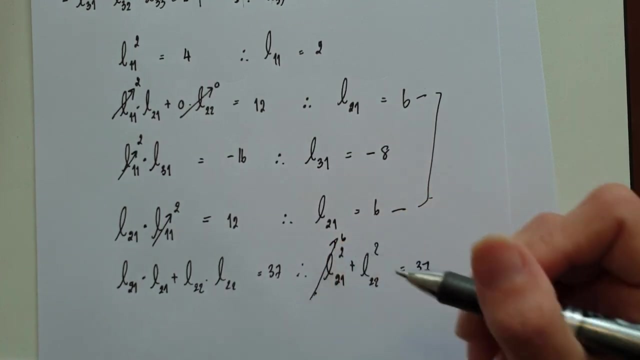 Here is L11.. L11 times L21 plus L22 times L22, equal to 37.. So here is L21 squared plus L22, squared, equal to 37.. And L21 is actually 6.. Right, Okay. So here is 36 plus L21.. 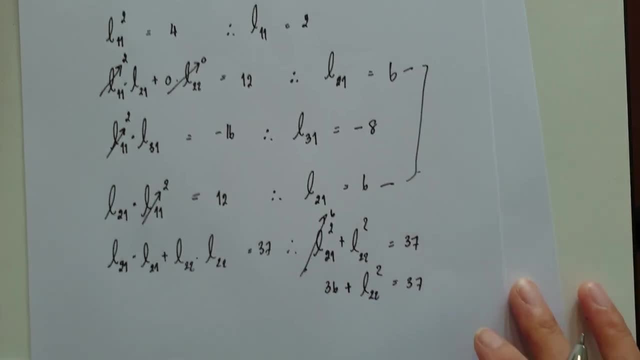 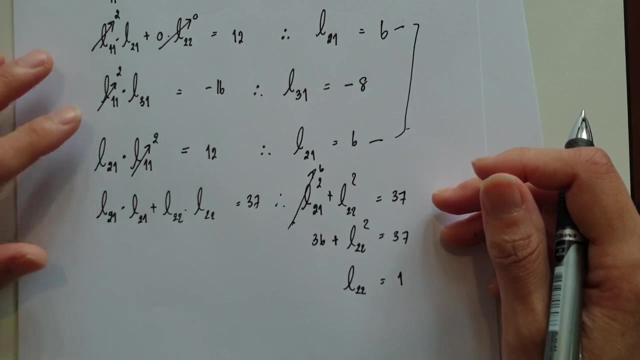 L22 squared equals 37.. So what I get is L22 is equal to 1.. Okay, And actually we already find L31.. We have to determine L32,, L33, right, So L32, we can calculate for L32.. 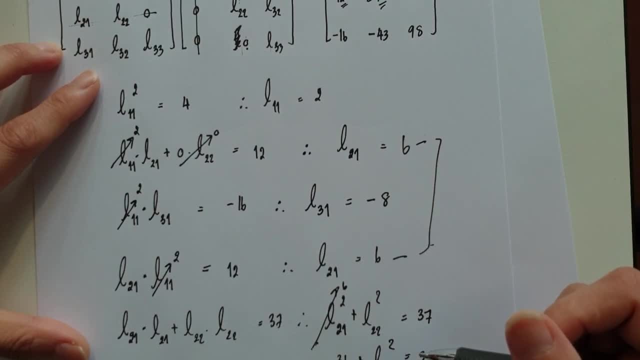 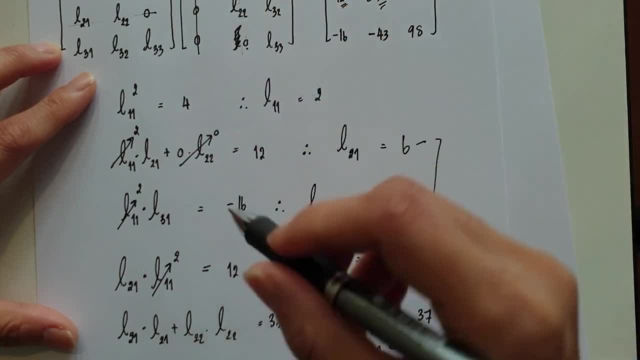 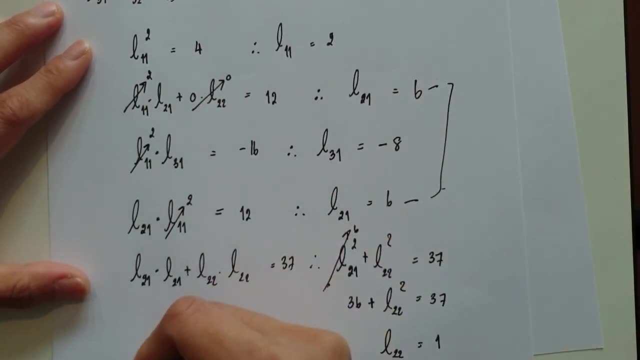 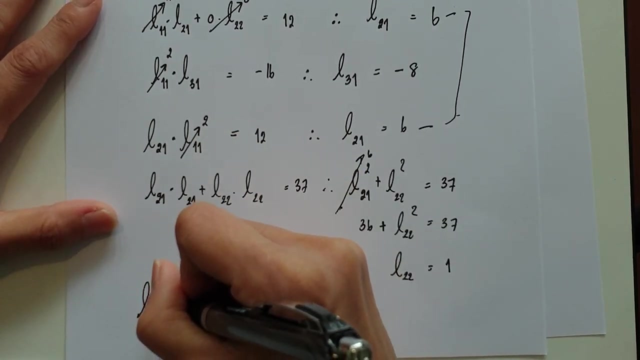 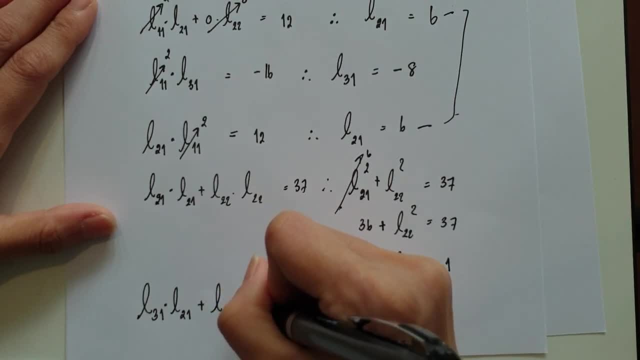 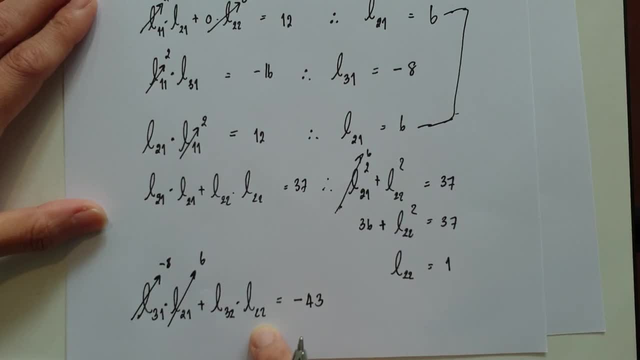 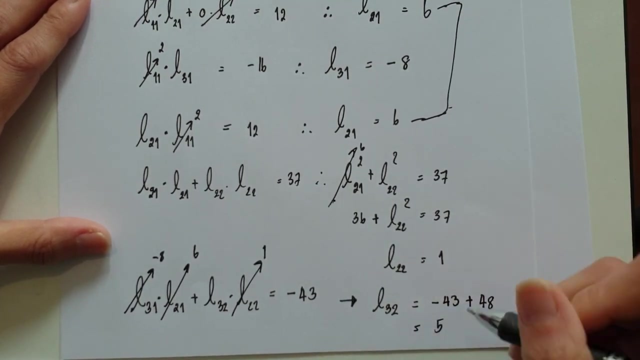 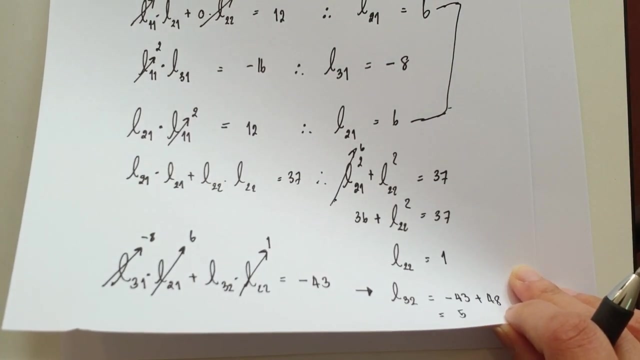 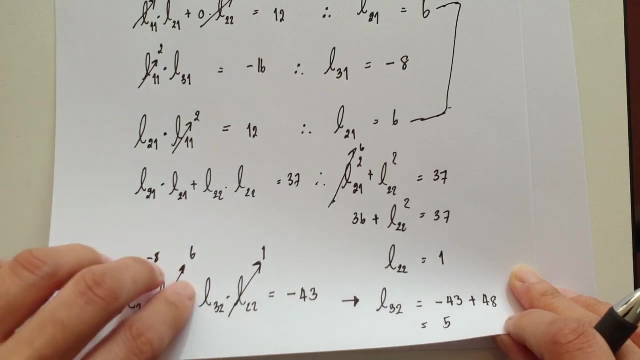 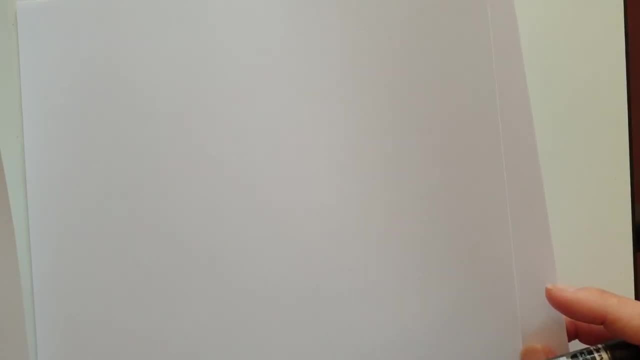 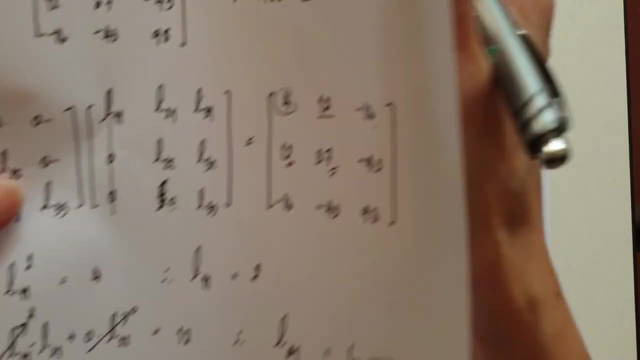 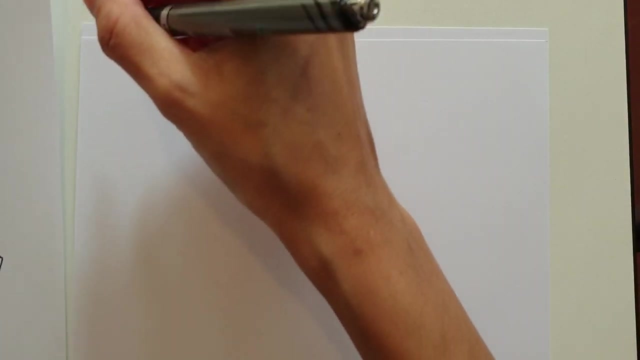 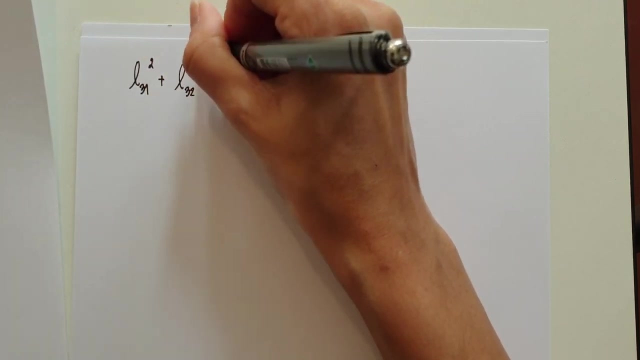 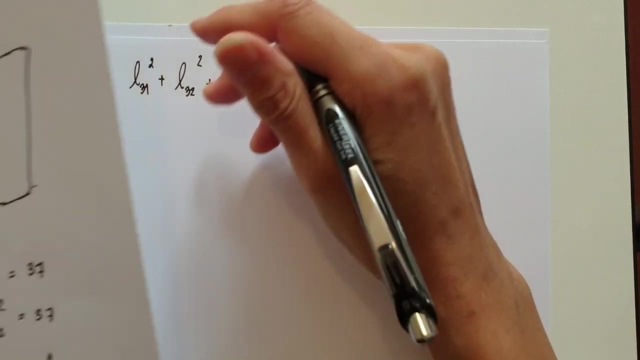 So R33 is R33 is actually- you can solve from here, multiply by here- equal to 98.. So it's actually R31 squared plus R32 squared plus R33 squared equal 98.. R31.. Okay, So R32 is 8, right. 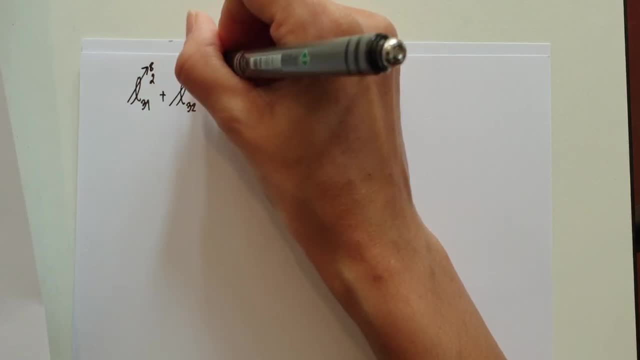 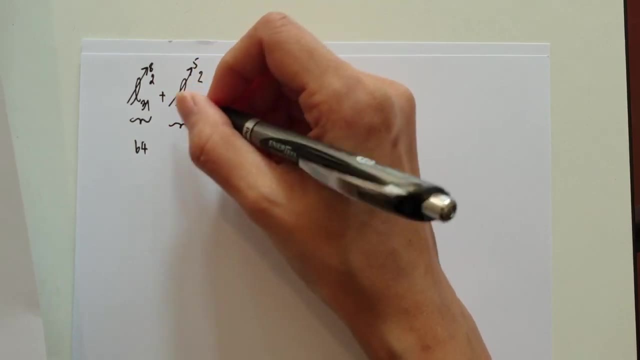 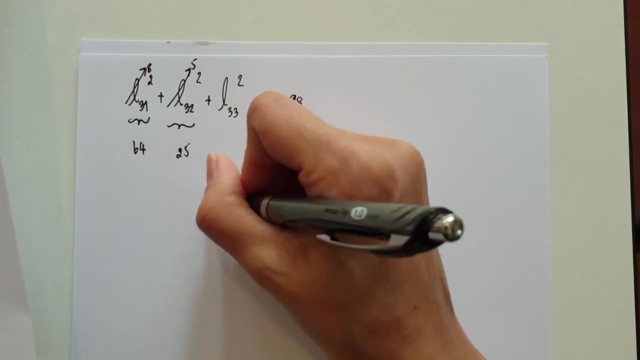 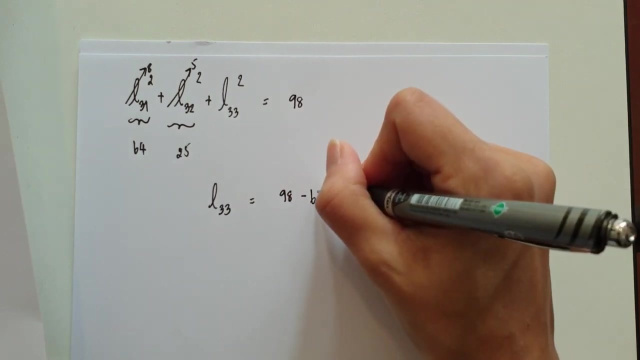 R32 is 5.. So here he got 40, 64.. 25 plus R33.. So what we get is R33 equal to 98 minus 64. So here he got 40, 64 minus 25.. 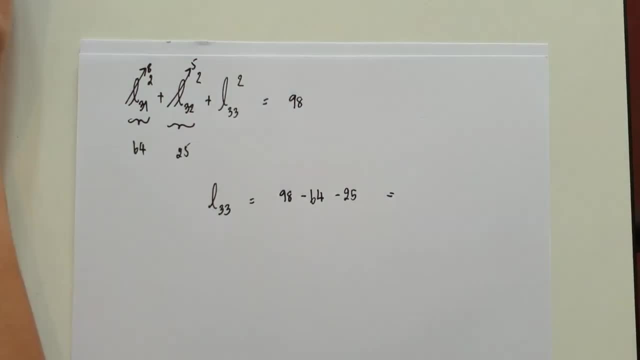 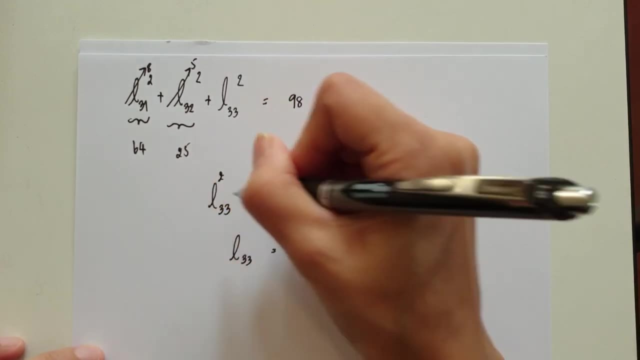 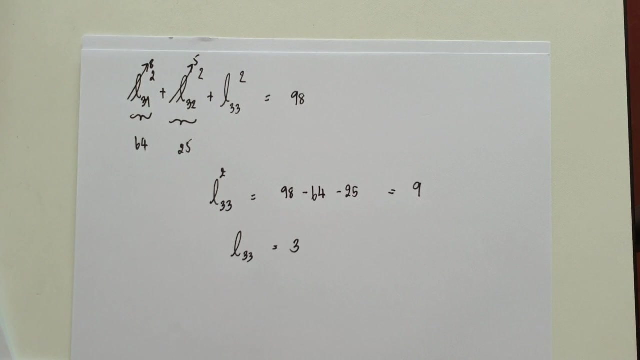 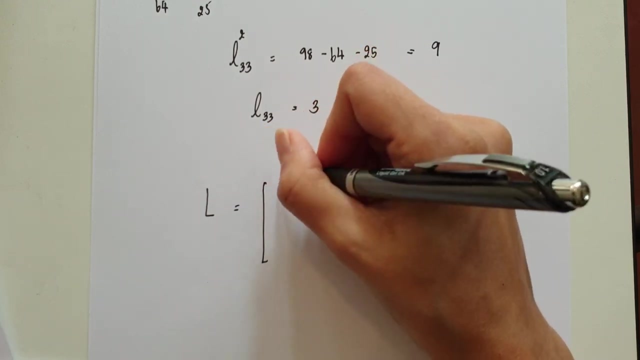 And it is equal to what? Equal to 9.. So R33 would equal to 3.. Okay, And finally, what we get is metric L. So L would equal to a metric of Q0.. So L would equal to L0.. 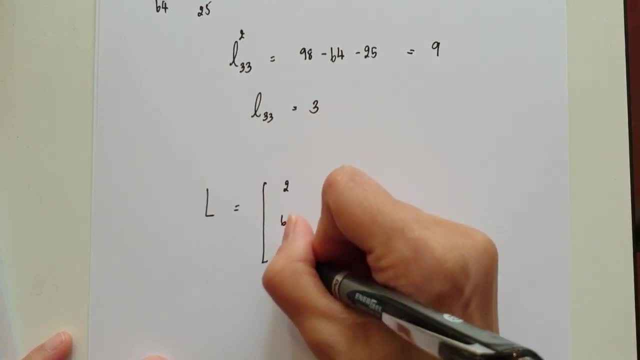 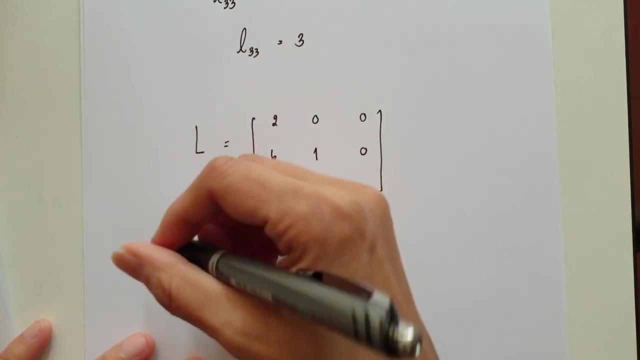 So X is equal to L0.. So X would equal to L0.. 6,, 1,, 0, minus 8,, 5, and 3.. So once we get out we go for the next step, Right. 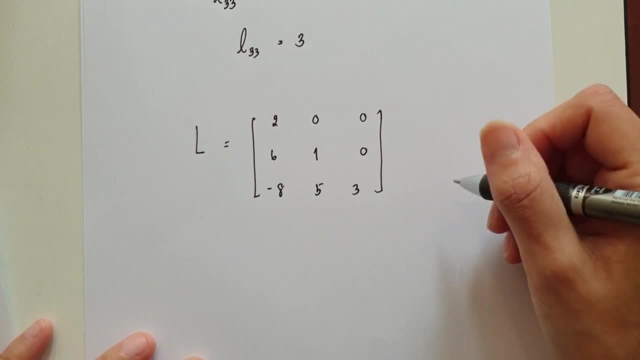 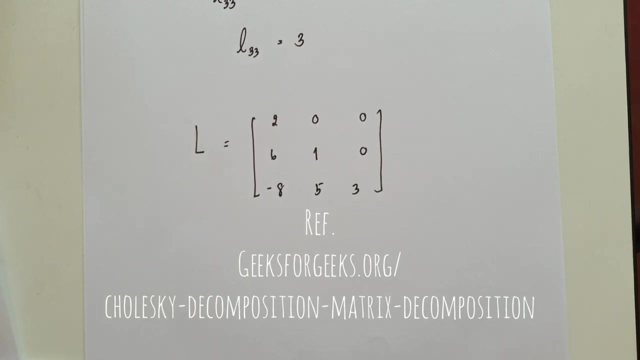 And I think you can follow how to solve the system of equation by Cholesky decomposition. So just this example would help you to figure out your equation, to find how we get the l matrix. okay, let's meet on the next session if you have any further question. 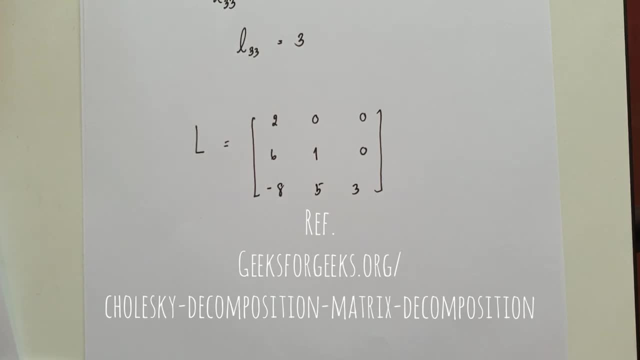 you can leave, take note and give it and we will have a discussion discussion time together. thank you,